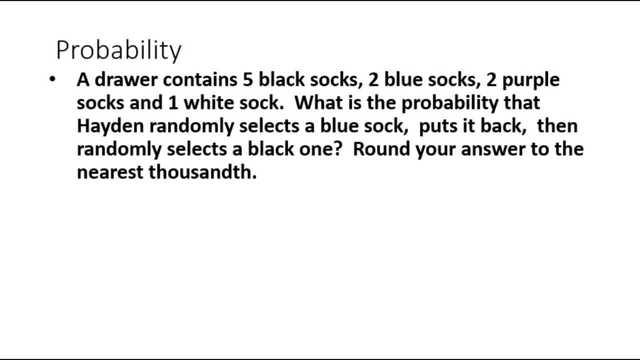 got a little bit here, Okay. so we've got our socks and we've got a blue one and a black one. So let's talk about the probability first, because he selected a blue sock first. Let's talk about what that probability is. So we've got and probability is. 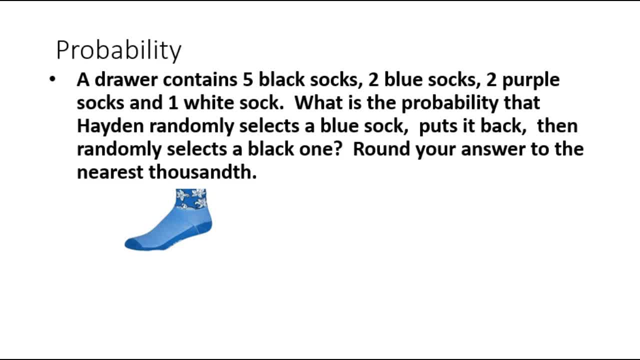 calculated when we talk about it, It's the number that we desire, in this case the blue sock, divided by the total number available or the total possibilities. So I have to add this up. I've got: 5 plus 2 is 7, plus 2 is 9, plus 1 is 10.. 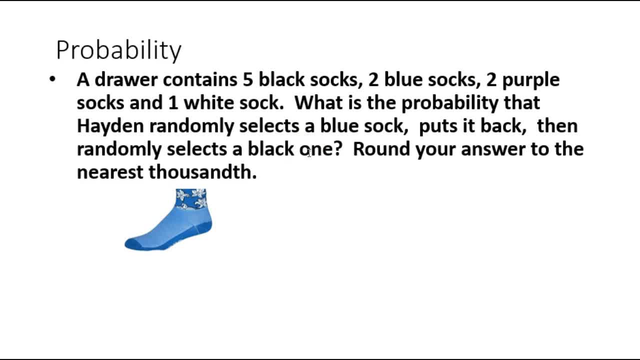 So it looks like there are 10 socks total. Hayden is going to reach his hand in there and pull one out. What's the probability? it's going to be blue. Well, there are two blue socks. That means we're going to go 2 divided by 10, or, if we reduce, it would be. 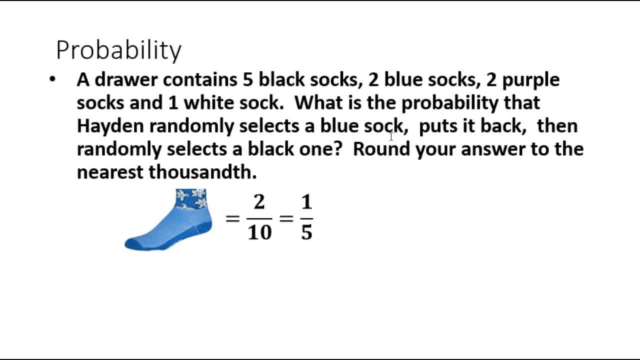 one-fifth. Okay, now he puts it back, then randomly selects a black one. Putting it back is a big. that's going to be important because if he puts it back now, we have 10 socks to choose from Again. if he were to have kept it, we would only have nine socks and that would 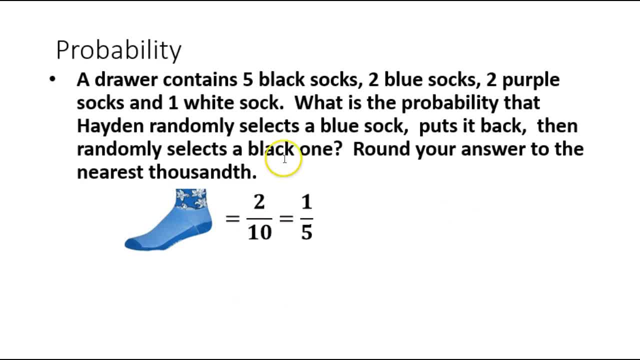 change our probability on our total possible on the black ones, But in this case he put it back. So we've got a black sock. now He put it back and then randomly selects a black one. He has five black socks available. So this is 5 over 10, which is one-half, and 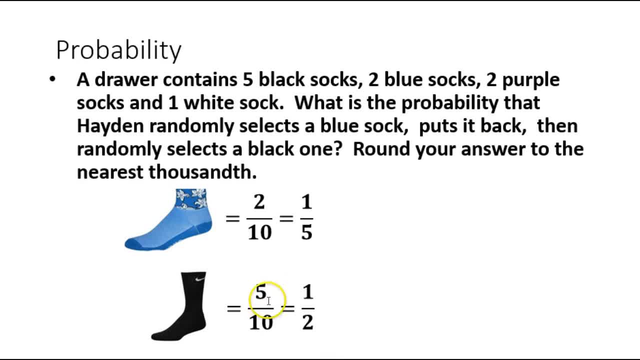 again. if he kept it, it would have been 5 over 9.. That's the only real big difference here, but he had 10 to choose from, because he put it back. Now we're trying to determine what the probability is that both of these events occurred. So when? 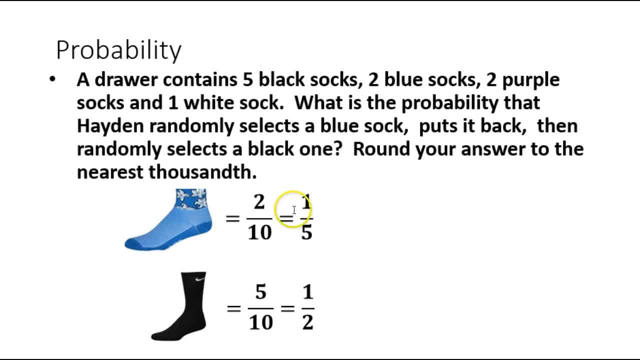 we're trying to figure out that probability. what we're going to do is multiply these two together One-fifth times one-half. Okay, so we go. one-fifth times one-half, that gives us one-tenth. We're asked to round our answer to the nearest thousandth. 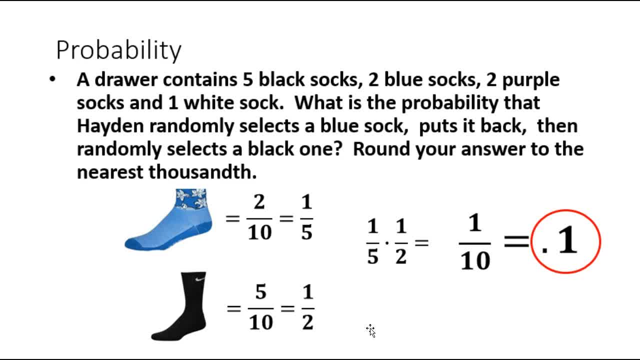 Thousandth is three decimal places, However, one-tenth is just .1.. That will work fine, So we just write it as .1.. If you wanted to, you could write .100, but it wouldn't make make much sense. It's just .1 would work just fine. on this one. 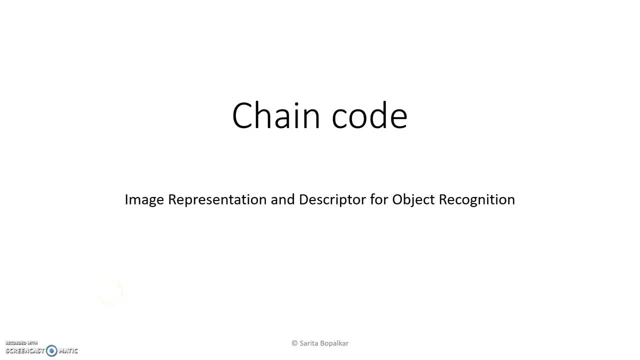 Hello and welcome. In this video, we are discussing chain code. And this is a technique in image representation and descriptor for object recognition. And here we start our machine vision system.